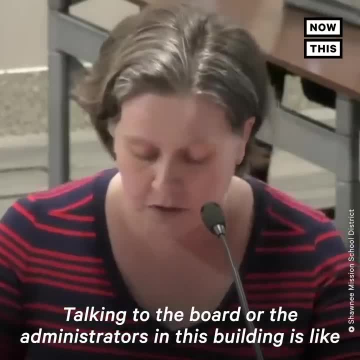 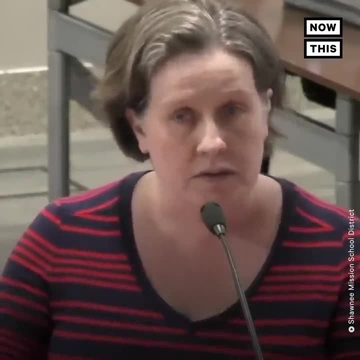 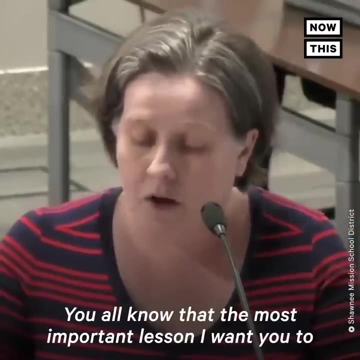 their teachers. Talking to the board or the administrators in this building is like shouting into the wind and I won't waste my breath, But I would like to address my students, many of whom are watching the livestream tonight. Alright, guys, you all know that, the most important lesson I want you to take away. 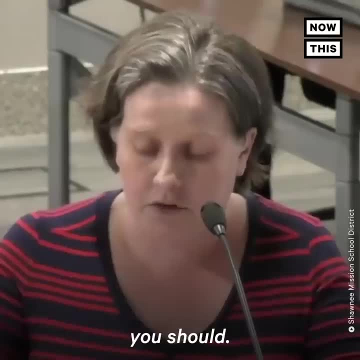 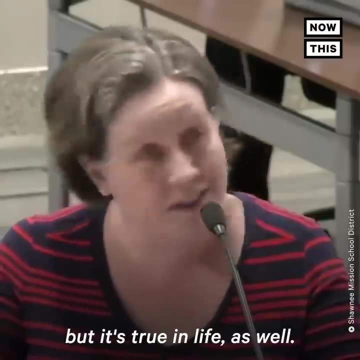 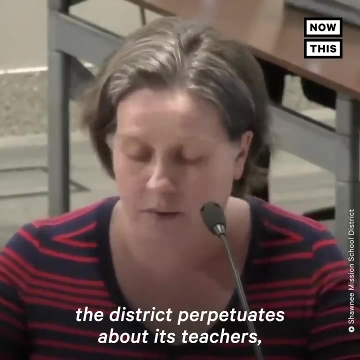 from your time with me is: just because you can doesn't mean you should. Usually, I'm applying that lesson to technology violations or intellectual bullying, but it's true in life as well. I could accept this contract, smile and stay silent about the lies the district perpetuates about its teachers. 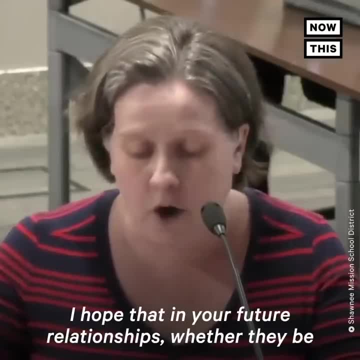 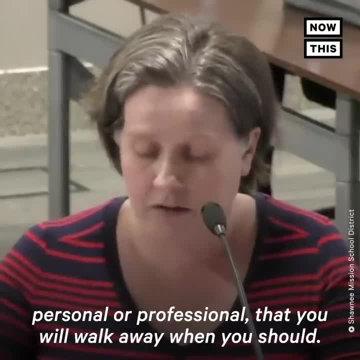 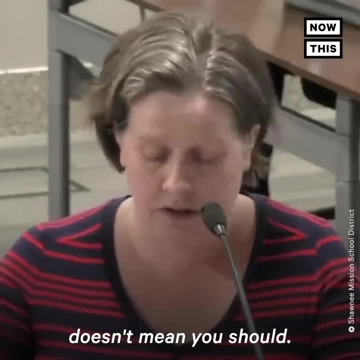 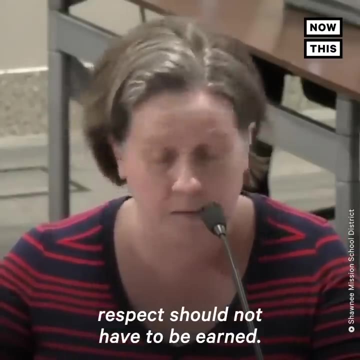 that in your future relationships, whether they be personal or professional, that you will walk away when you should. Just because you can accept less for yourself doesn't mean you should. Here's another important lesson: Despite what you may be told, respect should not have to be earned It. 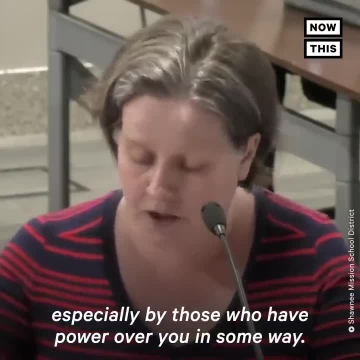 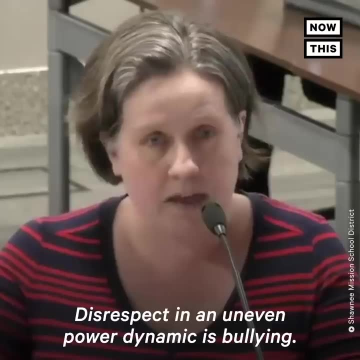 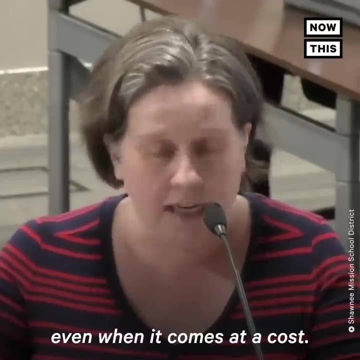 is owed to you as a human being, especially by those who have power over you in some way, in an uneven power dynamic, is bullying. when we see bullying, we must stand up and call it out, even when it's hard, even when it comes at a cost, just because you. 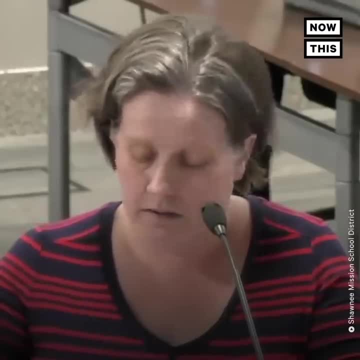 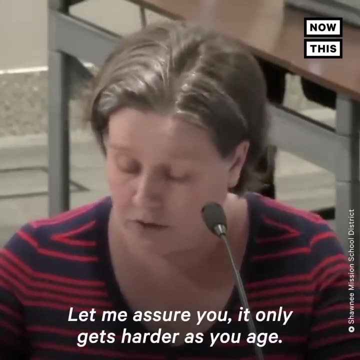 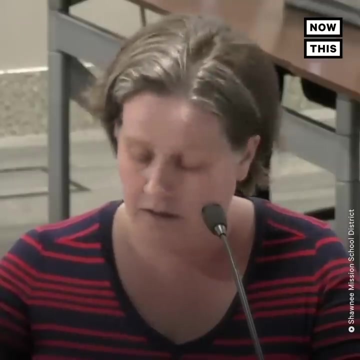 could stay silent doesn't mean you should. starting over is never easy. you eighth graders know that well as you prepare for high school. let me assure you it only gets harder as you age. but just because you can stay in a familiar place doesn't mean you should go chase your dreams, find your passions, remember. 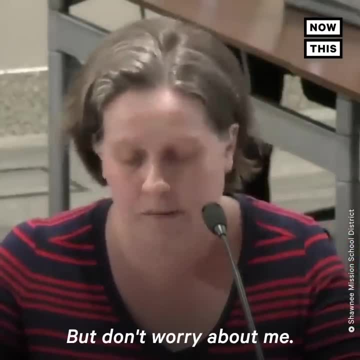 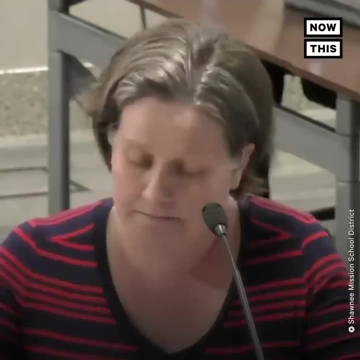 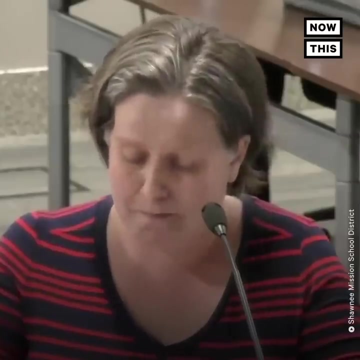 me and your acceptance speeches. but don't worry about me, I'm a highly educated, very talented teacher. they are in high demand right now in other districts. and finally, I don't know what I'll be doing when the bell rings at 8: 40 tomorrow morning. but I won't be greeting you with the hallways, please. 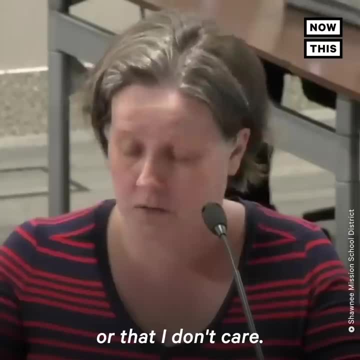 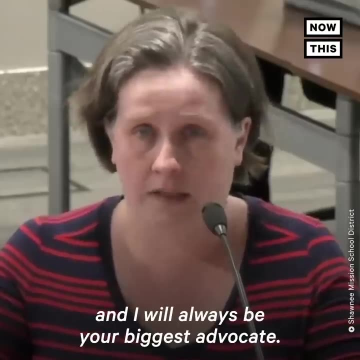 don't see me. my empty doorway is a sign that I've abandoned you or that I don't care. that empty doorway is my sign that you are still my favorite humans and I will always be your biggest advocate. there will be no clarifying questions. I don't.